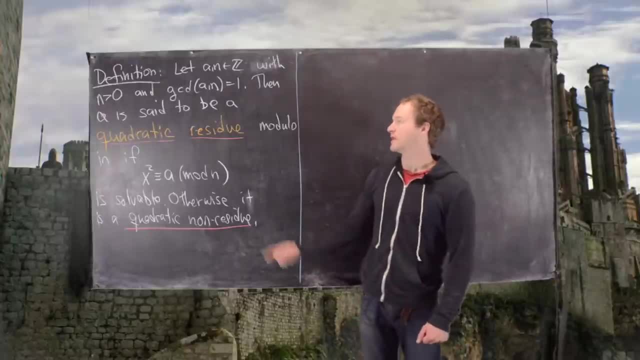 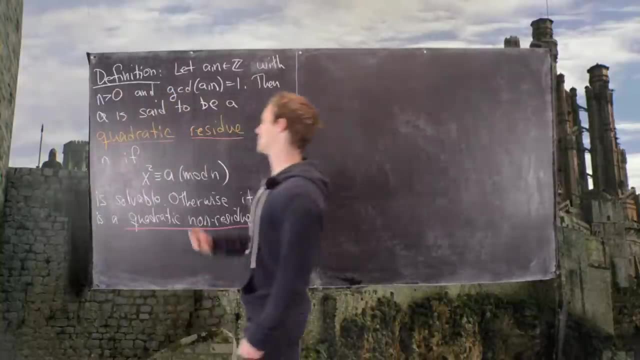 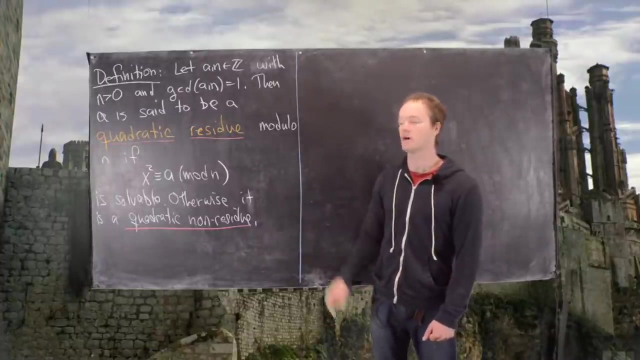 and the gcd of a and n is 1, so they're coprime. then a is said to be a quadratic residue. modulo n, modulo n: if x squared congruent to a mod n is solvable. So if it's not solvable we call it a quadratic non-residue. 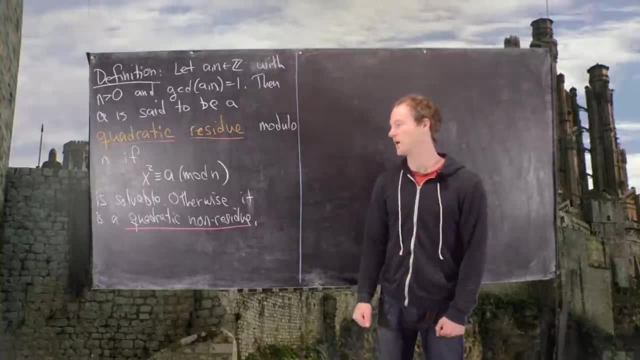 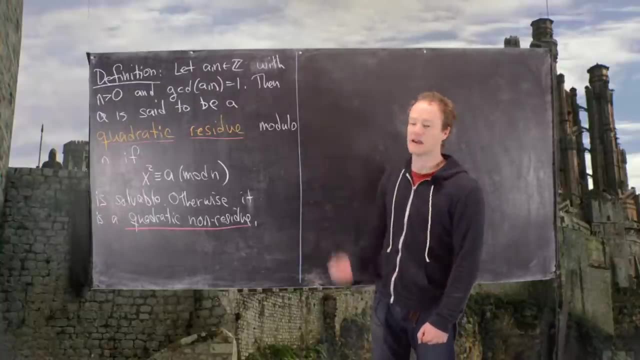 And just as a note in general, we're going to be proving quite a few results based on this notion of a quadratic residue, and we'll mostly be interested when n is an odd prime. Okay, so let's look at an example. 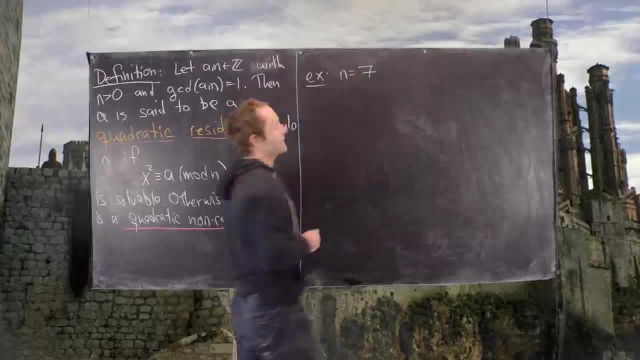 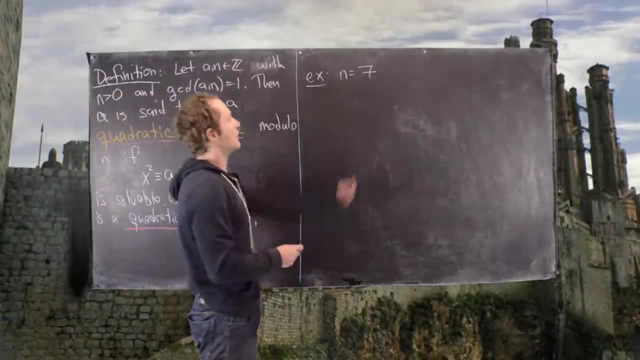 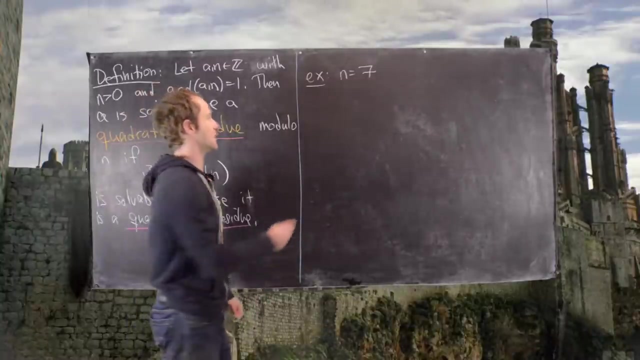 So let's say n equals 7, so that's obviously an odd prime. so this would be one of the cases that we'll be proving results about later. So now what we're going to do is just square all of the numbers mod 7 and see what the outputs are. 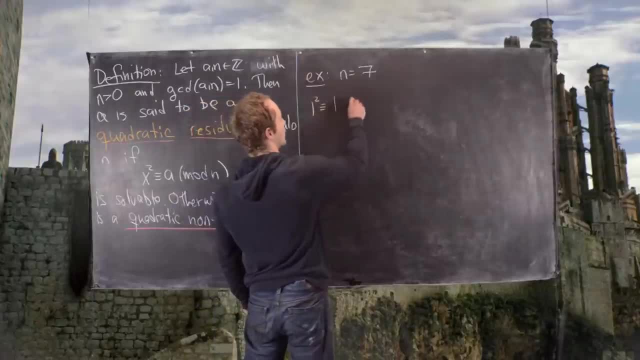 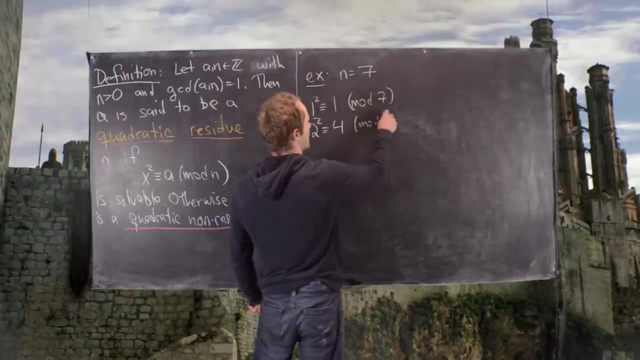 So if we take 1 squared, so that's obviously congruent to 1 mod 7.. 2 squared, that's obviously congruent to 4 mod 7.. 4.. 3 squared, so that's equal to 9, which is congruent to 2 mod 7.. 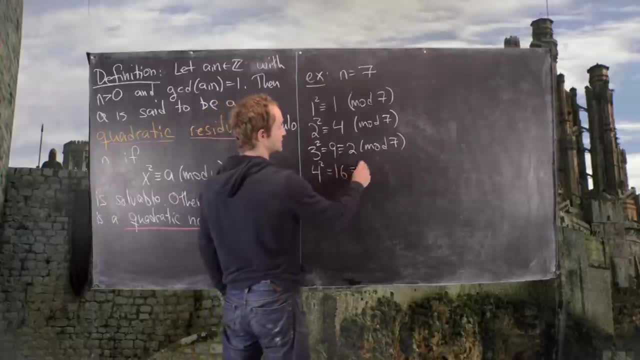 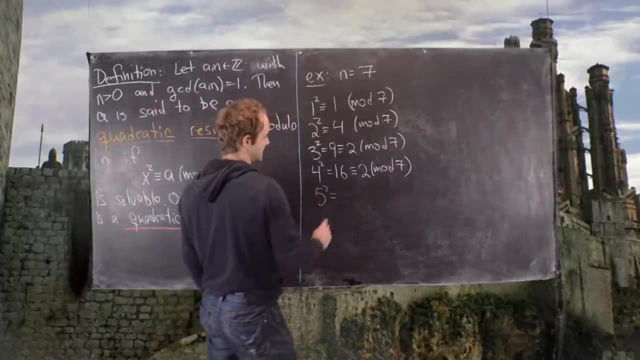 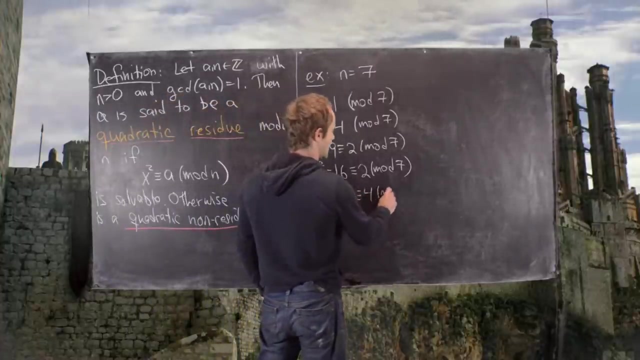 4 squared, that's equal to 16, which is also congruent to 2 mod 7.. So 5 squared is equal to 25.. 25 is 4 more than 21,, so that is 4 mod 7.. 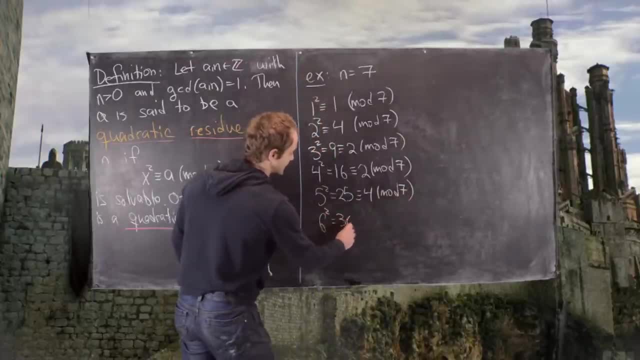 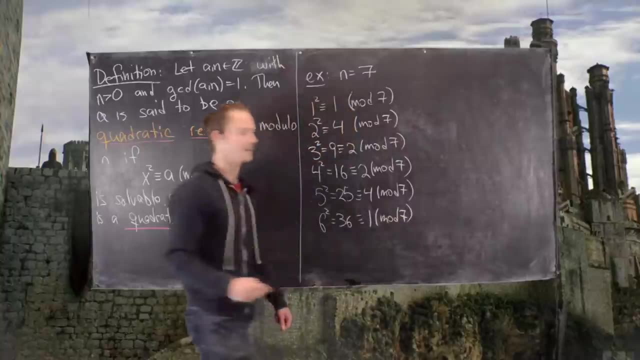 And then finally, 6 squared is equal to 36.. So that's equal to 36.. Which is 1 more than 35, and that is congruent to 1 mod 7.. Good, so, look, there's some nice structure here. 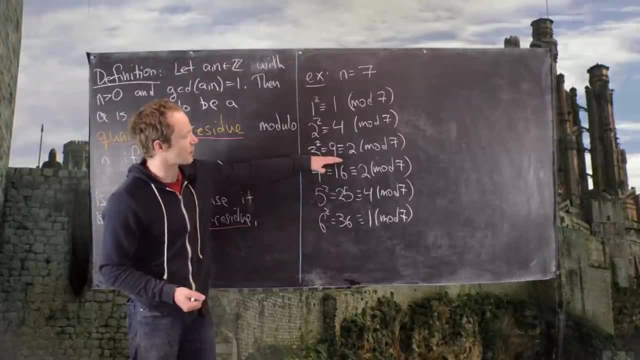 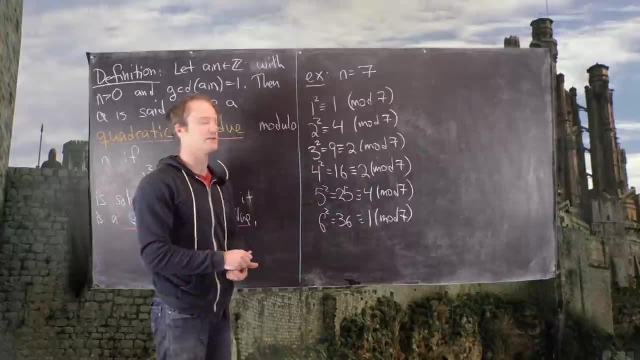 And in fact, like if we fold this list over this line, right here they match. So 2 matches with 2,, 4 with 4, and 1 with 1.. So again, this will be as part of some of the results that we prove a bit later. So now, what I want to notice here is that we can do invert, all right. So we can do invert and then invert again. So we can do invert and then invert again. So we can do invert and then invert and then invert again. 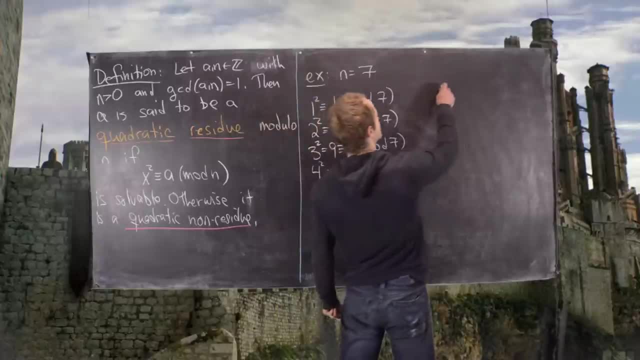 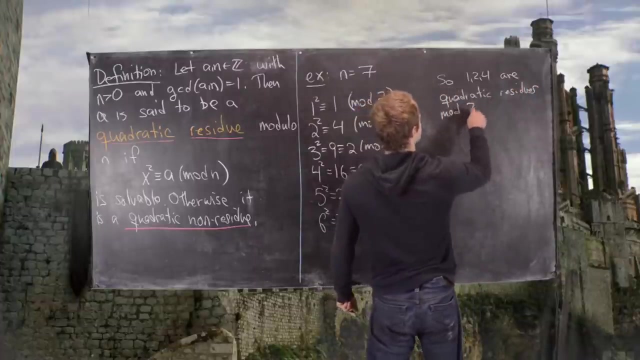 So we can do invert and then invert again, list all the quadratic residues and all the quadratic non-residues. So let's see 1,, 2, and 4 are quadratic residues, Mod 7, so that's the first thing that we can say. 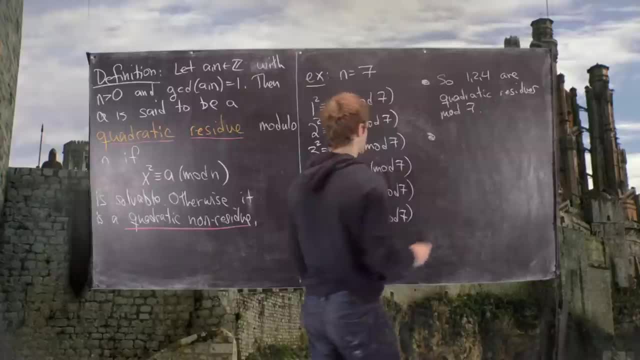 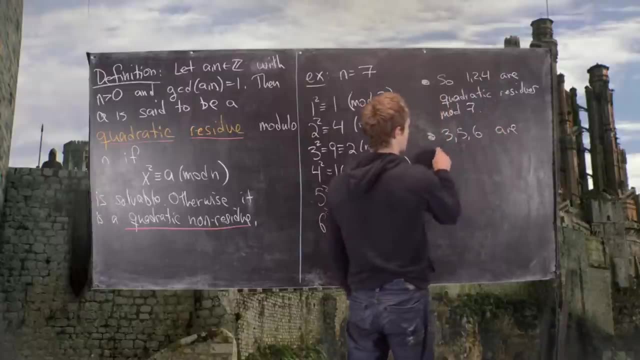 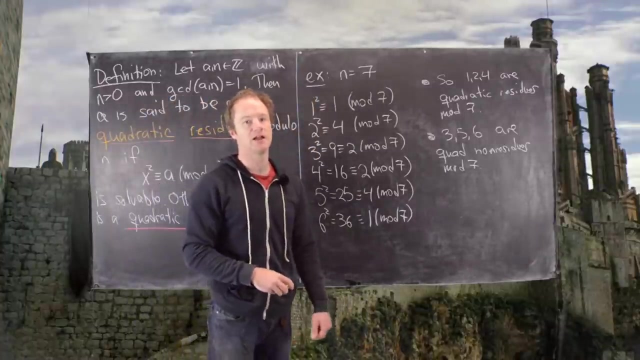 The second thing we can say is: let's see whatever's left. so which is 3,, 5, and 6 are quadratic non-residues, Mod 7.. Okay, good, So we've looked at an example where we have an odd prime, and so now I'm going to do one. 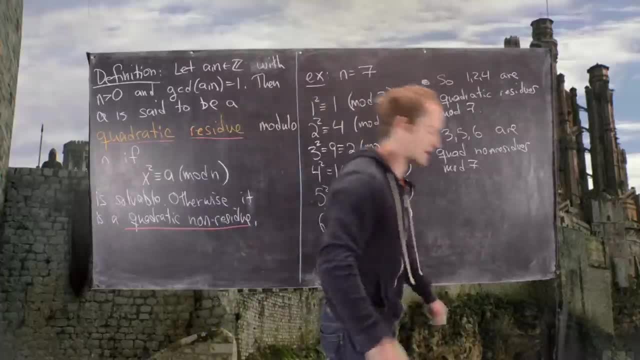 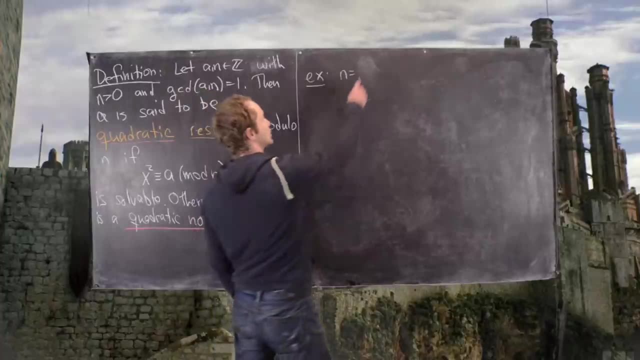 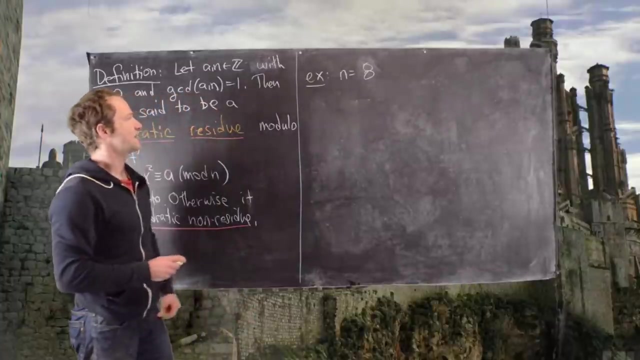 more example where we have a composite number, just for good measure. Okay, So we're going to look at another example of quadratic residues. This time we're going to look at modulo 8.. We're going to use the same strategy, So we're going to take all of the numbers that are relatively prime to 8 and square. 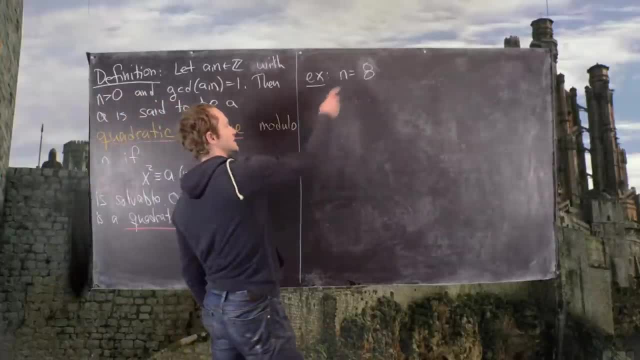 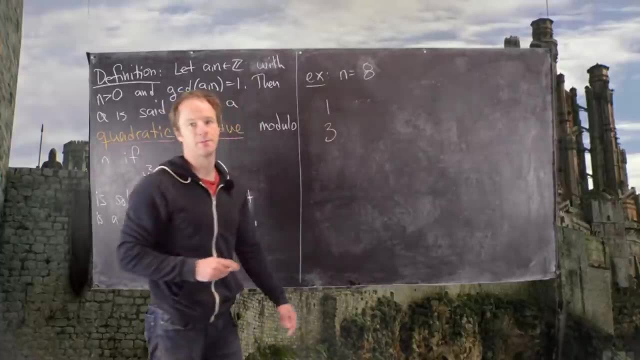 them and see what we get. So let's see: what do we need for relatively prime numbers? first We need 1, so 2 is not relatively prime, so we can't use that. 3 is, 4 is not, so we can't. 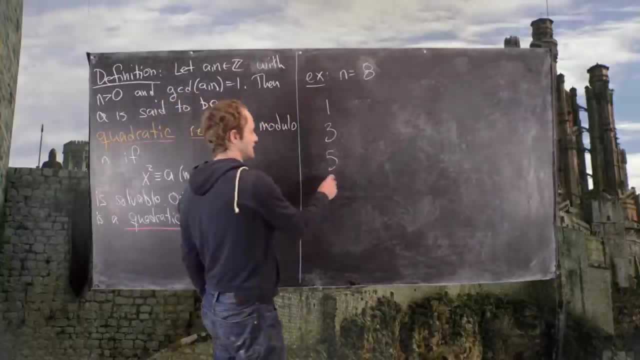 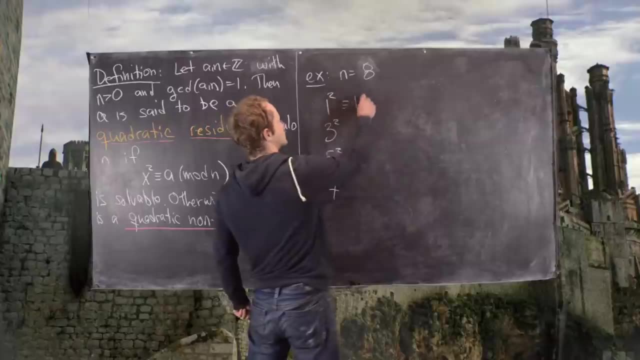 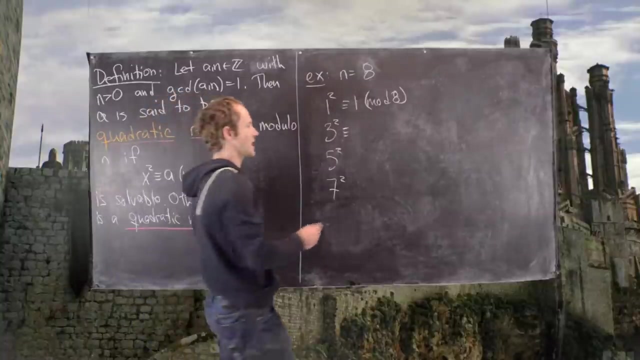 use that 5 is, 6 is not And then finally 7 is. So these are the squares that we need to calculate. So 1 squared is obviously congruent to 1 mod 8, 3 squared is 9, but 9 is 1 mod 8, 5 squared. 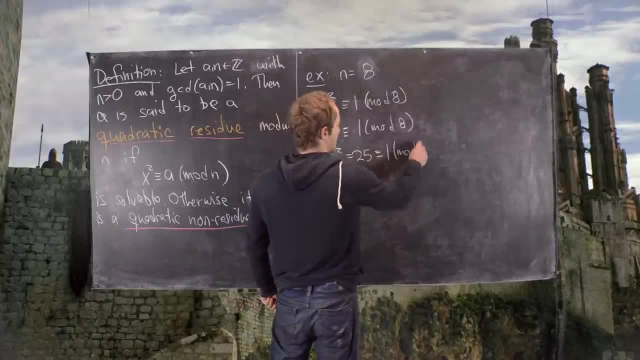 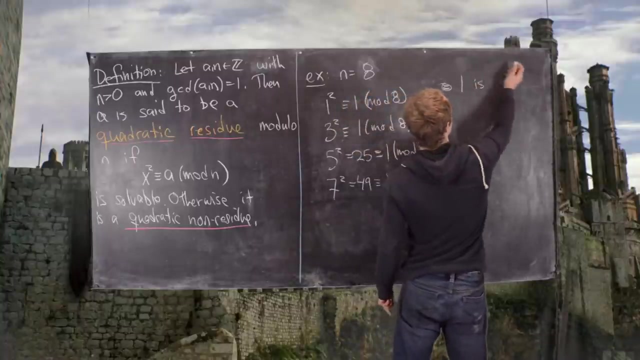 is 25, which is again 1 mod 8, and then finally, 7 squared is 49,, but that's also 1 mod 8.. So what that tells us is that 1 is the only quadratic residue modulo 8.. 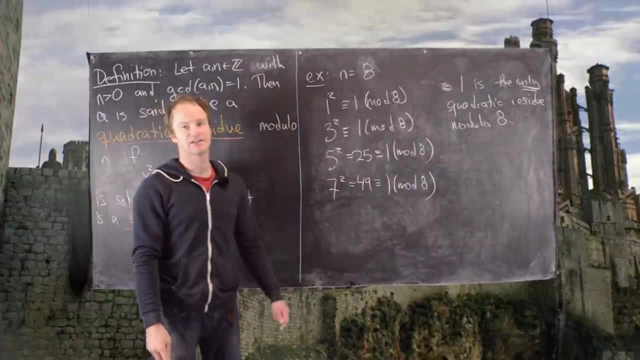 So we have 1 as a quadratic residue. that means 3,, 5, and 7 are quadratic non-residues. Okay, That's the end of the video. in the next video we're going to prove a couple propositions. regarding quadratic residues.